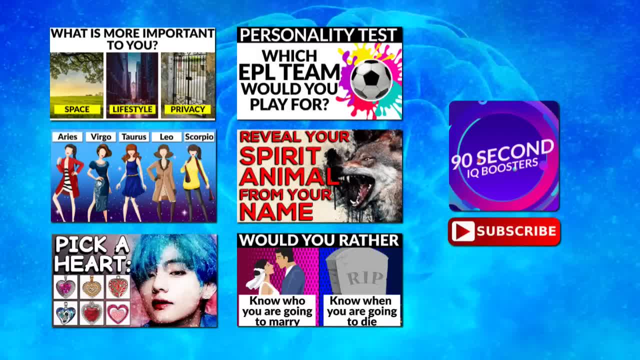 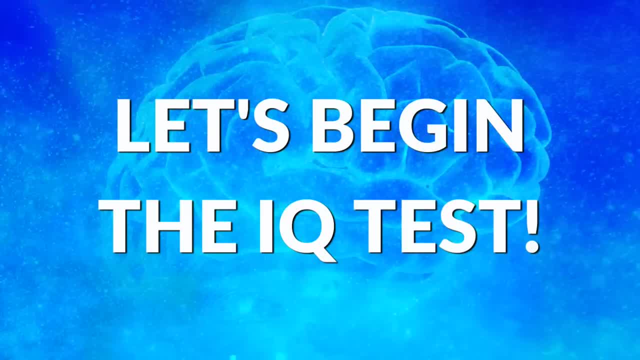 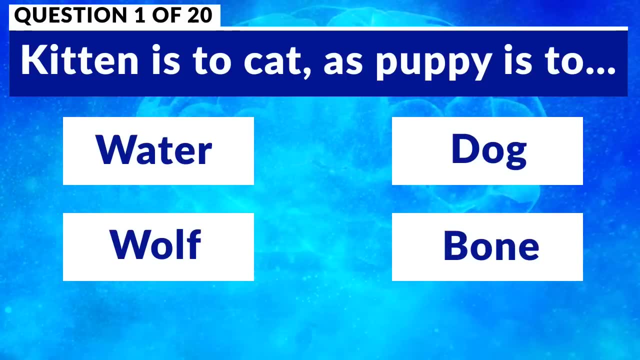 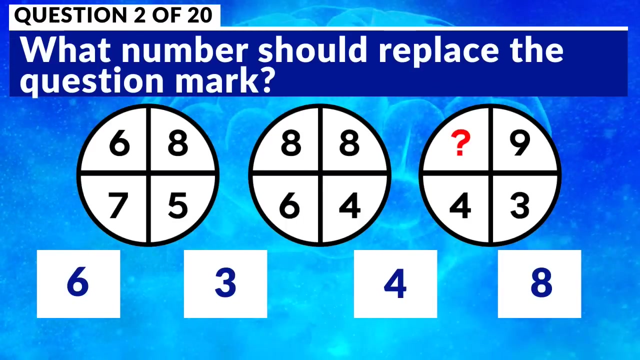 with the IQ test. please take a moment to subscribe to 90 Second IQ Boosters for more interesting IQ tests, personality quizzes and more. Let's begin the IQ test. What are your IQ levels? 1., 2., 3., 4.. 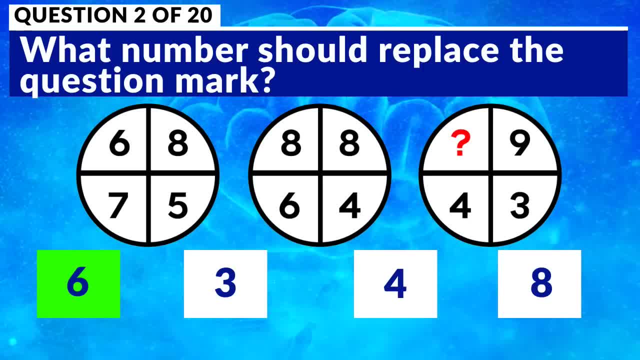 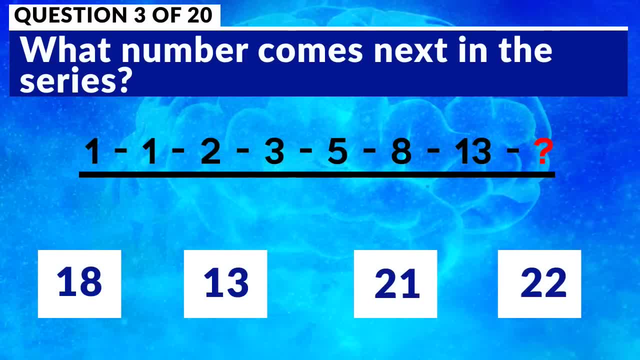 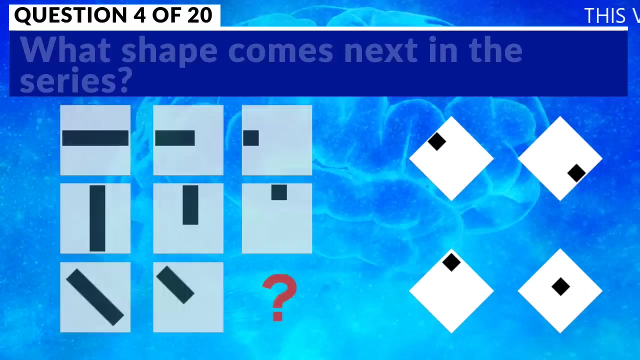 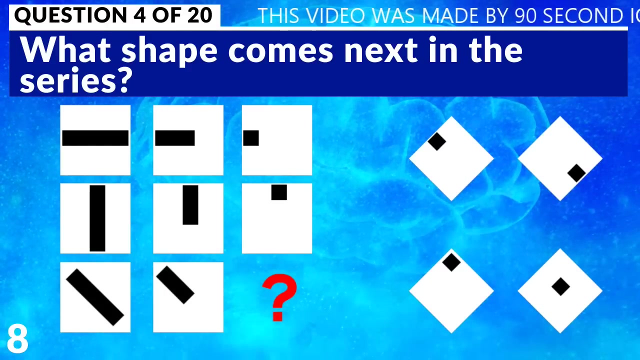 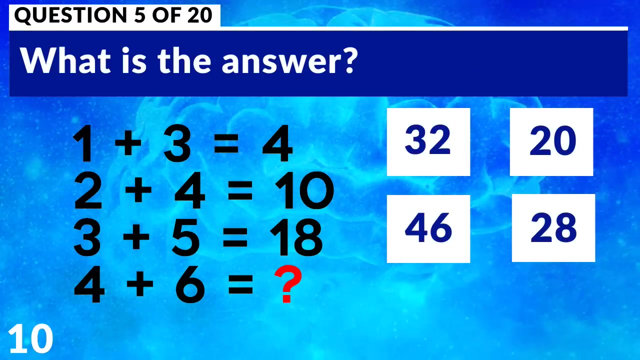 5., 6., 7., 8., 9., 10., 11., 12., 13., 14., 15., 26., 22., 23. 32.. Thank you, Thank you.